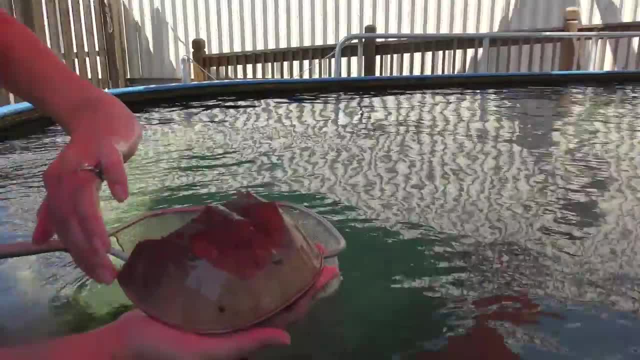 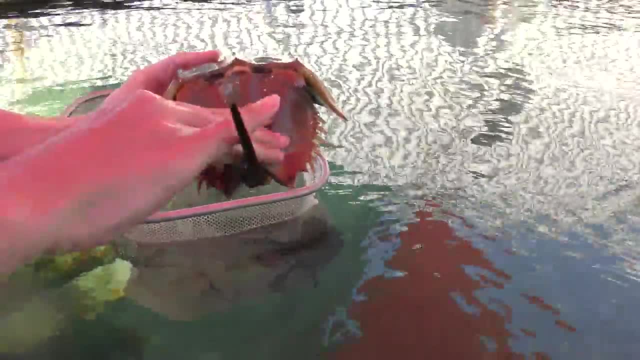 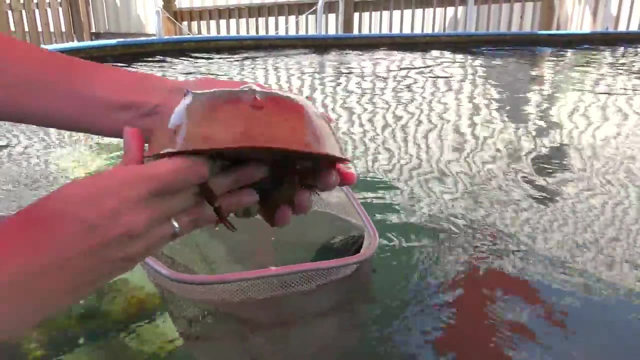 the overall structure of the horseshoe crab. the main parts of the body are the head, which is also called the prosoma, and the abdomen, the back part, which is called the epistisoma, and the tail or the telson, And some of the cool features of horseshoe crabs. if you look right on they have. 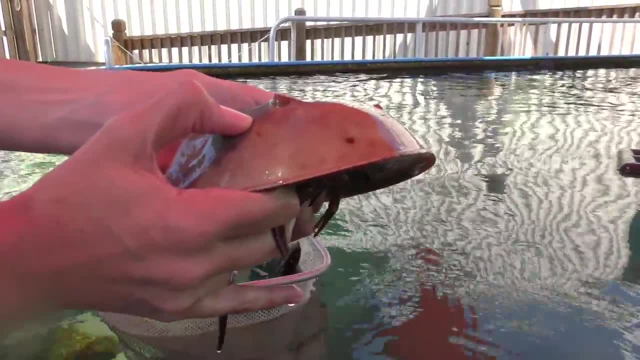 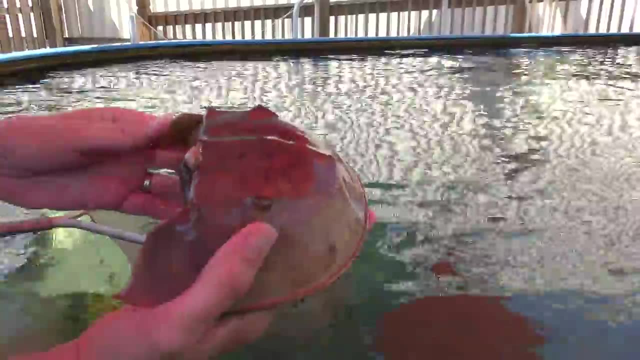 a really cool compound eye that you guys might be able to get a good look at there. Very often horseshoe crabs are covered with other kinds of organisms that live on the surface, and we'll see that in a minute when we pull out the male. 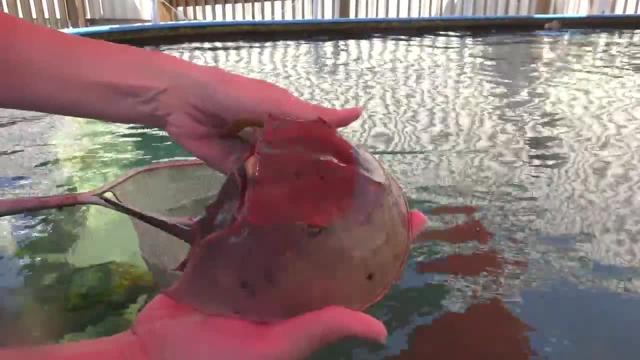 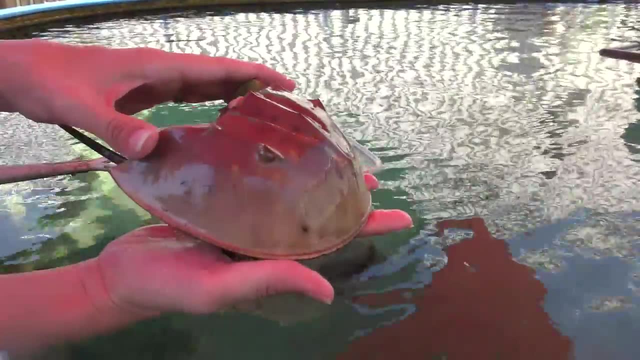 But this female. she's pretty clean and pretty slick. Horseshoe crabs have a really amazing immune system so they're able to fight off a lot of types of diseases and infections And actually their blood is used as the gold standard for testing all medical supplies. 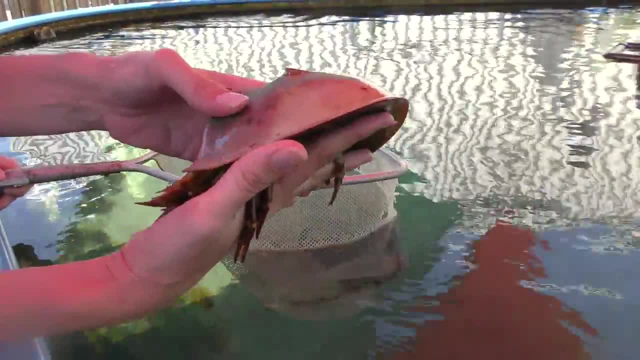 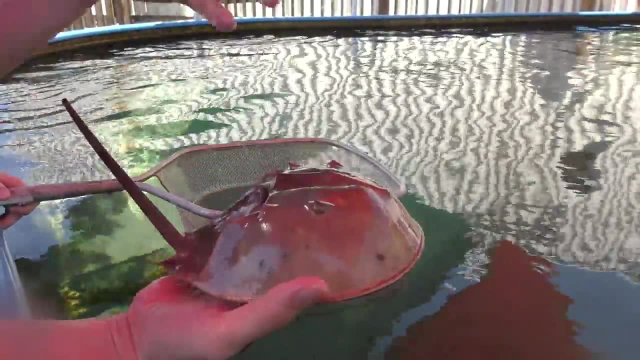 and equipment that we use. So if you've ever had an injection, for example, of a drug, or you've ever had stitches, any of those products were tested with horseshoe crab blood to make sure that it's safe to be used on humans. So they're really, really important to us. 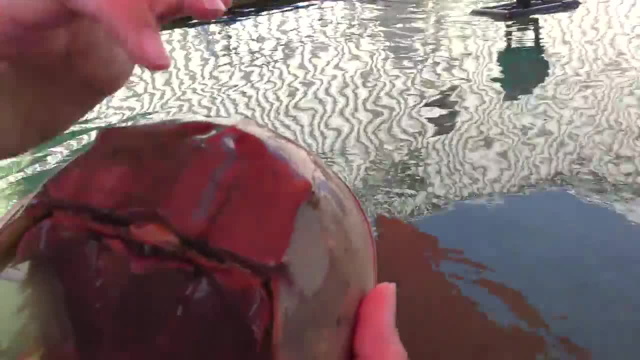 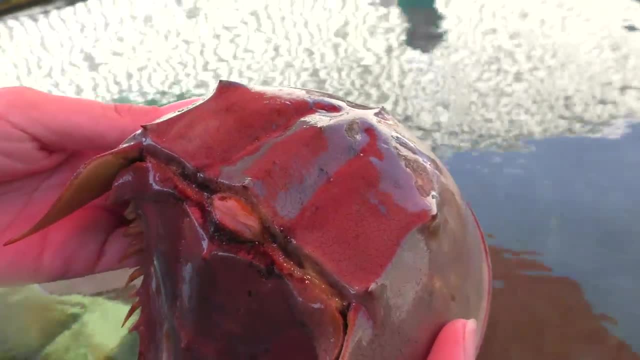 And if you want to look right here at the hinge area that's actually right under there is the heart, which is where they take the blood that's actually used to make the compounds that are important for protecting people. So we're going to go ahead and turn this girl over. 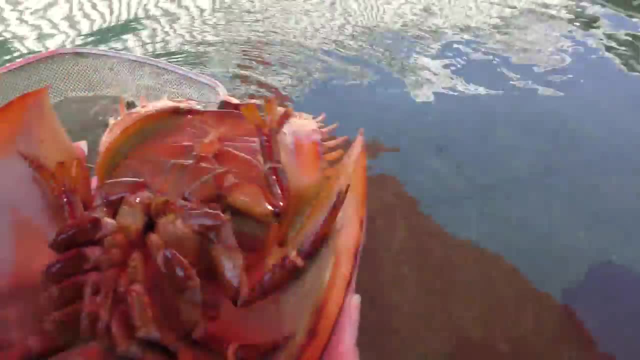 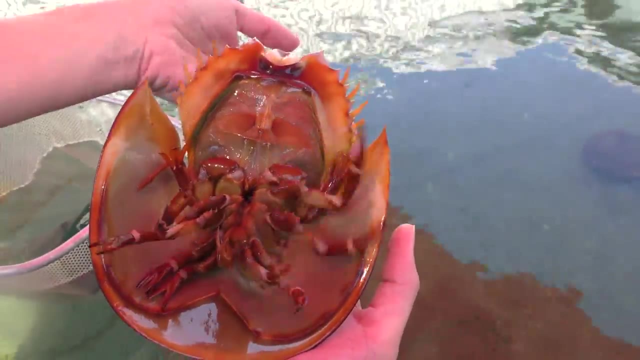 And now we're looking at the underside of her And you guys will notice that I'm holding her by her head or her prosoma, And that's the best way to hold a horseshoe crab. You don't want to pick them up by the tail because you can really hurt them if you pick them up by the tail. But 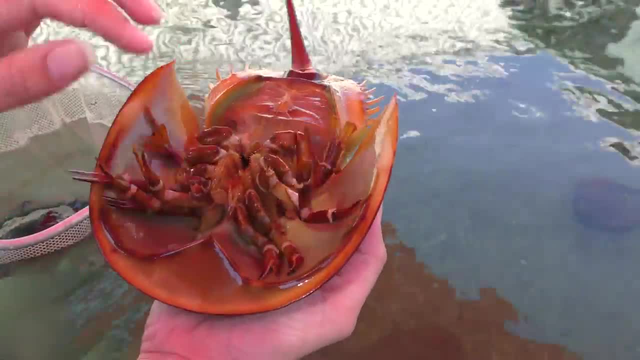 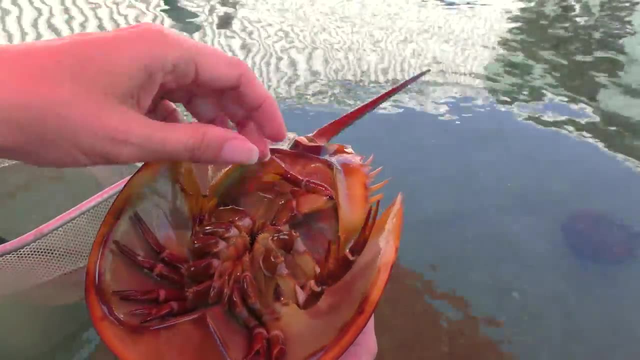 you hold them like this and you can really get a good look underneath. So what we're looking at is all of her legs And she's got some walking legs. but you'll also notice she's got these really cool looking pusher feet And these kind of look like flowers And those are used for pushing and 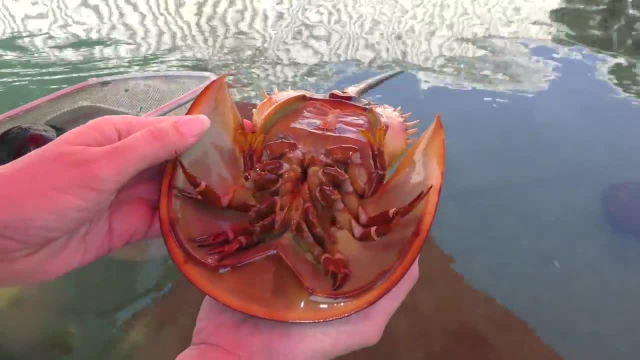 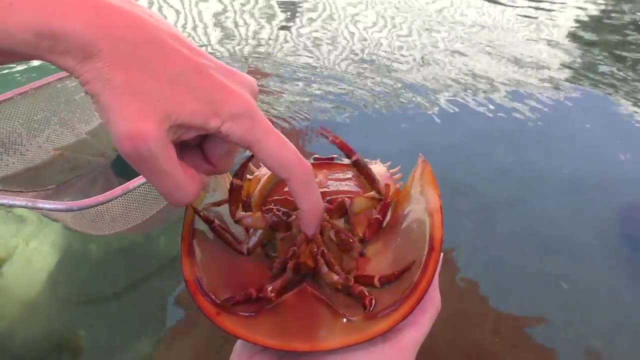 digging into the sand, because they will bury themselves, for example, to build nests when they want to lay their eggs in the sand. And right in here in the middle, at the base of the legs, these are called the nathobases because they're used for actually chewing, And that's the mouth. 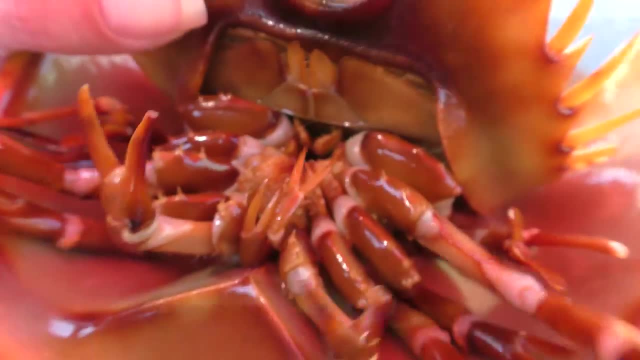 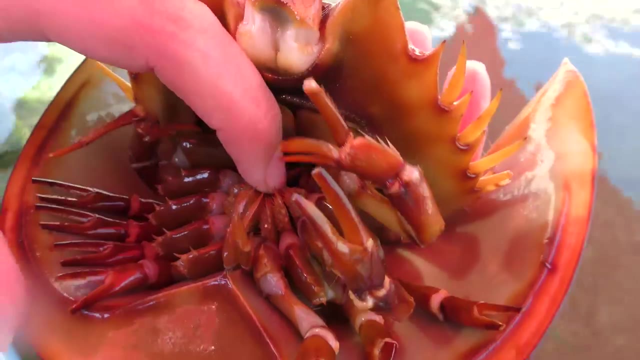 inside And so you can see they're really kind of hairy. All those hairs have a lot of sensors in them that are used. It's like a big tongue, And then they'll rub those legs together at the base to pull in food and to kind of macerate food or grind it up a little bit as they're eating. 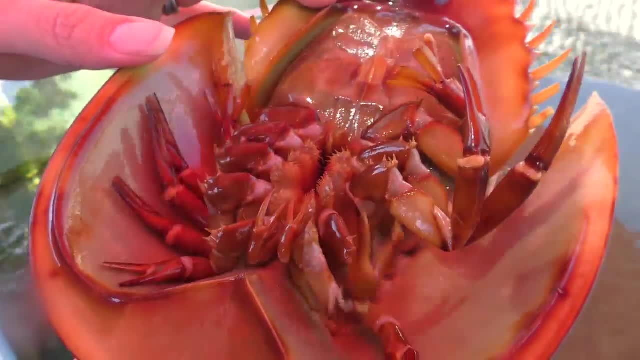 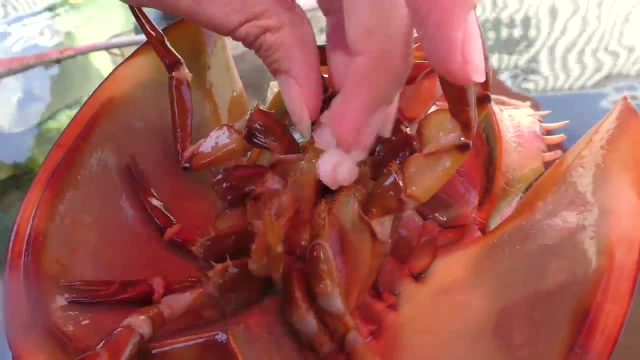 So they'll pull it right in there. But she's all clean, so you can see all of her hairs and everything So cool. And we'll go ahead and see if she wants to take a little bit of. it's a weird way to eat, but we'll see if she wants to take a little food in. 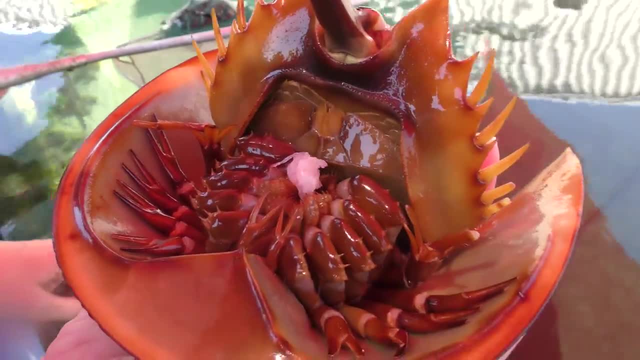 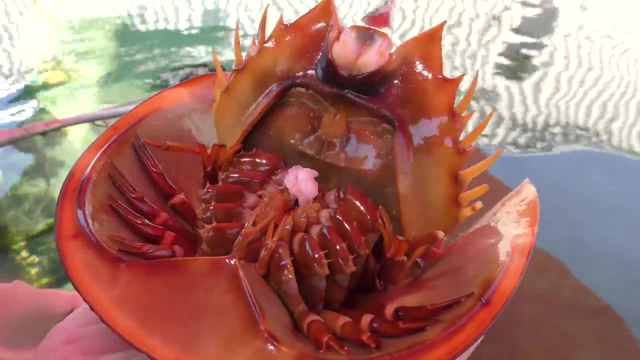 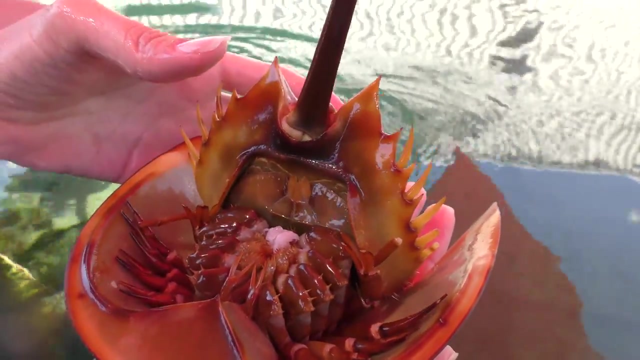 She smells it and decides to take it in. And if you look just behind the legs she's kind of curled up on us now. This is a defensive maneuver that crabs do. If you look behind the legs you'll see all of these little folds here Underneath. there is where she has her gills. 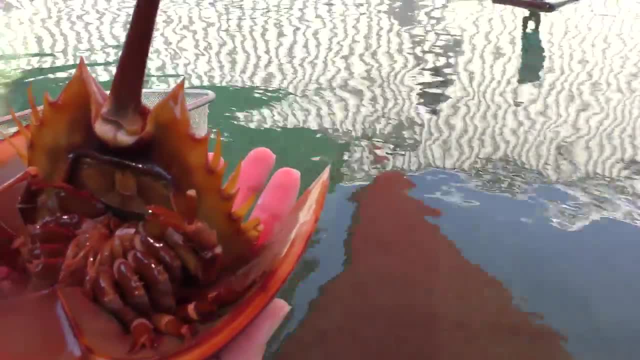 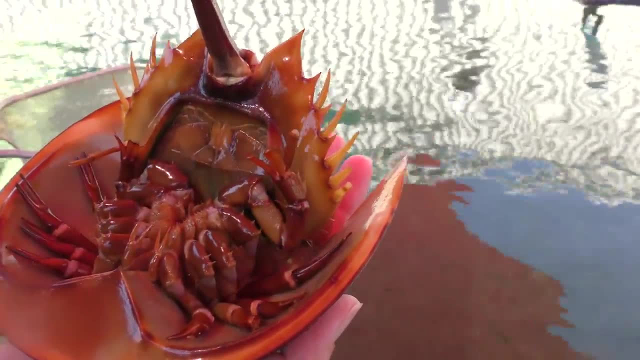 Oh, look at that. She's taken the food in. Good girl, Like a little vacuum cleaner Out in the wild, these animals will eat any kind of thing that's in the sand. They sort of act like little vacuum cleaners, So as they. burrow through the sand. they'll actually take in their food, but they'll also take in the sand itself and they'll kind of clean particles from the sand And then when they release their feces they sort of are releasing that clean sand that's been cleaned of all the organics. 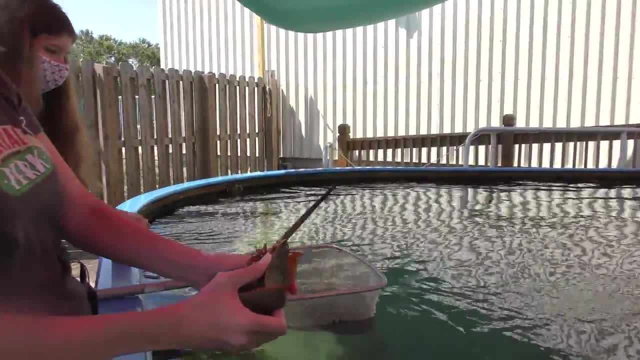 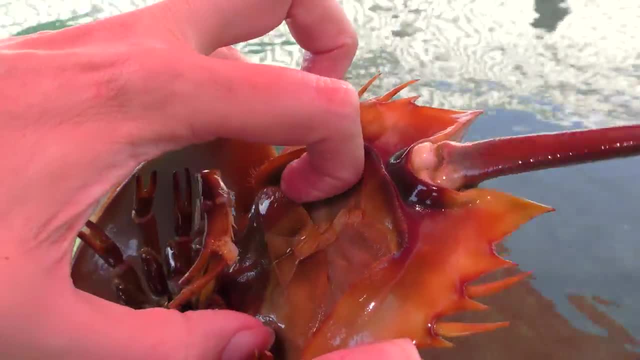 All right. So let's look underneath and see if we can get a good look at her gills under here. So the gills are how they breathe And if we just look under these flaps, she may not want to show us today The first flap. 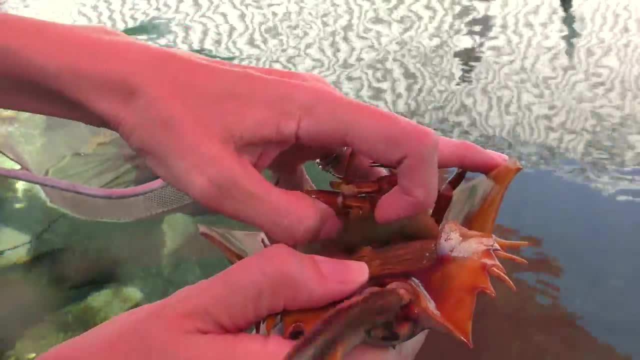 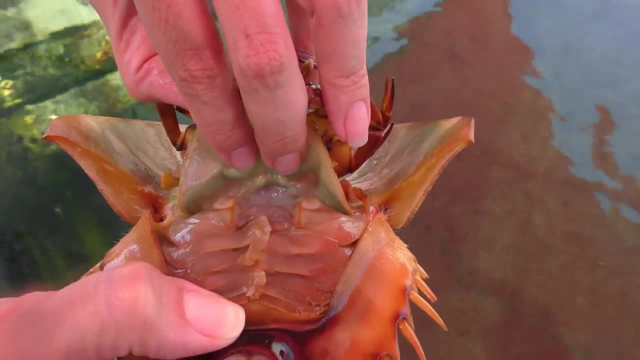 we also want to be gentle so we don't hurt her at all. The first flap is actually where they have their reproductive parts. So if you can see those two slits down there, that's actually how we know a male from a female, because the female has these broad slits to release eggs And a male 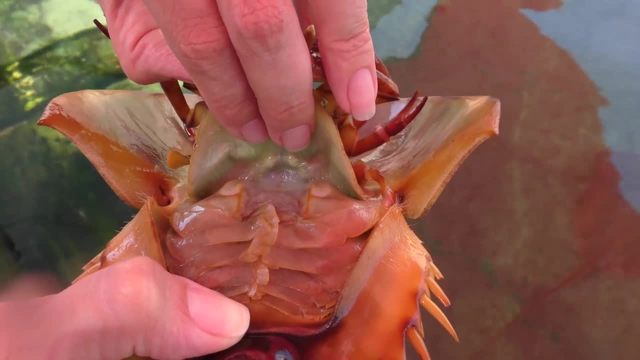 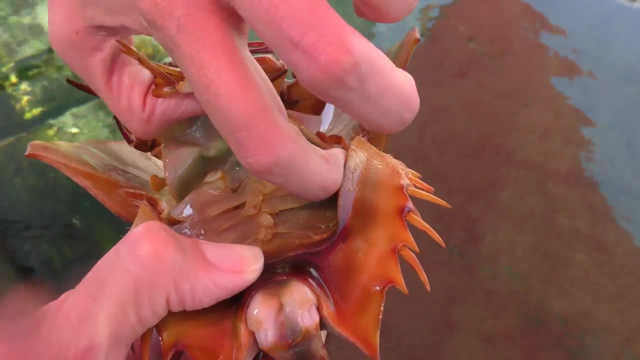 has little points where he will release his sperm or melt. And so hers right there, her two little slits where she releases eggs, And then behind that these are called the book gills, And I'm going to put her in the water and see if she'll flap her gills a little bit. Sometimes she will. 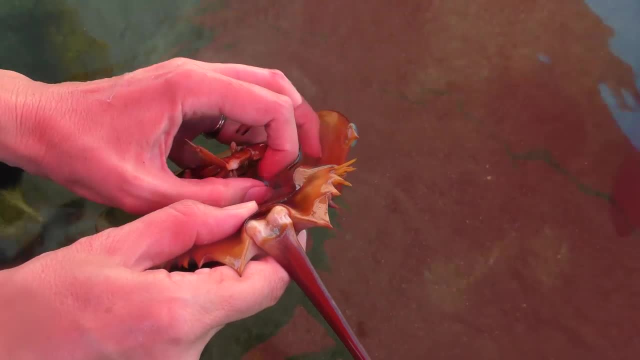 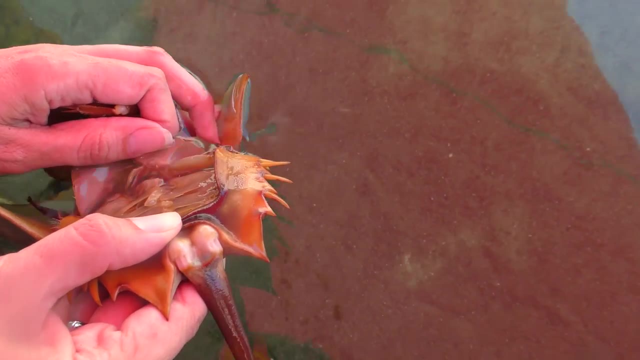 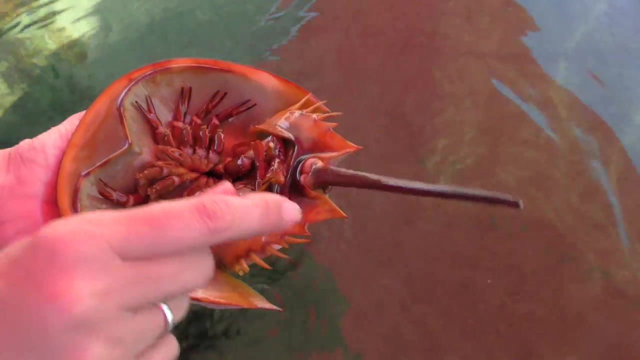 But if we open these up a little bit, you'll be able to see all the little flaps. underneath. There we go. All those little flaps are the gills that they use for breathing. So they're all underneath here, And then, last but not least, right under the tail here. guess what that is? 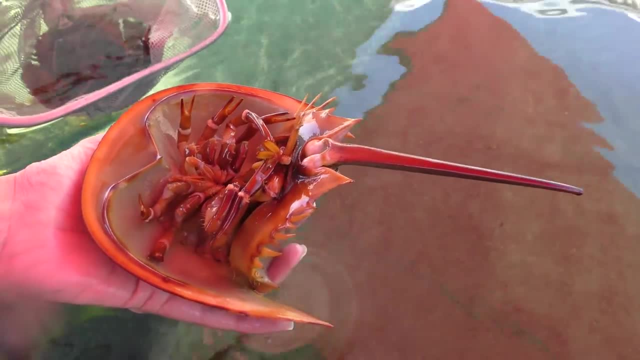 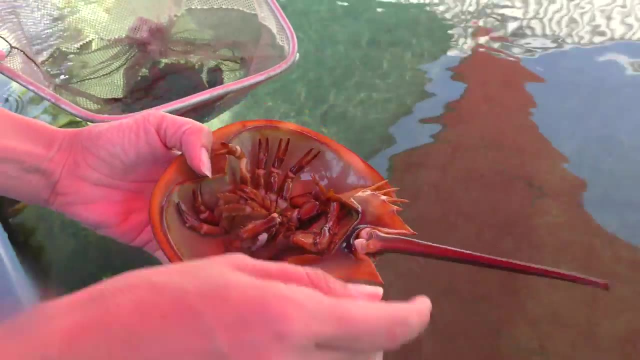 Beneath the tail. Yes, What's beneath the tail? That is where the waist comes out. That's where the waist comes out, right, That's the anus. There we go. Very good, All right, We'll go ahead and flip her back over A couple of other things. 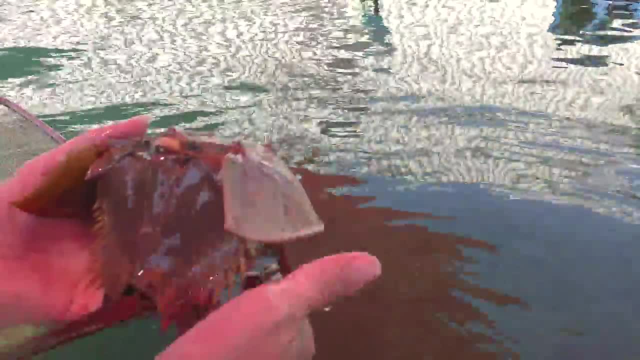 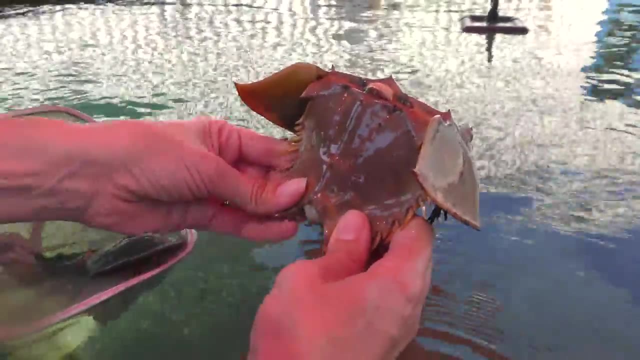 to notice on the female. Now this is a young female, so she doesn't have a lot of mating scars. But the males will clasp on to the back of the female. You can kind of see these two little marks here And I'll show you the claspers on the male in just a minute. But the male will clasp on. 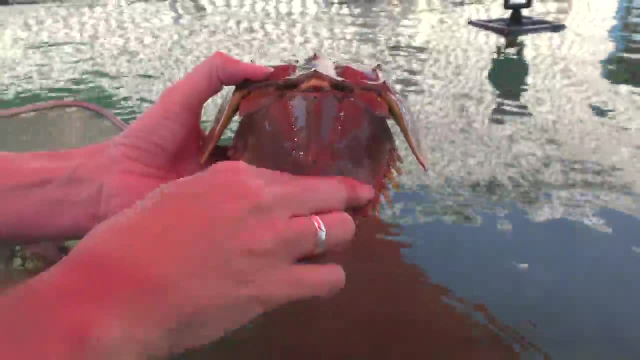 and hold on to the female for mating, And so she'll usually get some scars along here where his shell has rubbed into her shell, And you'll also. I want you to notice the front of her shell and the back of her shell, And then you'll also notice the front of her shell as well. 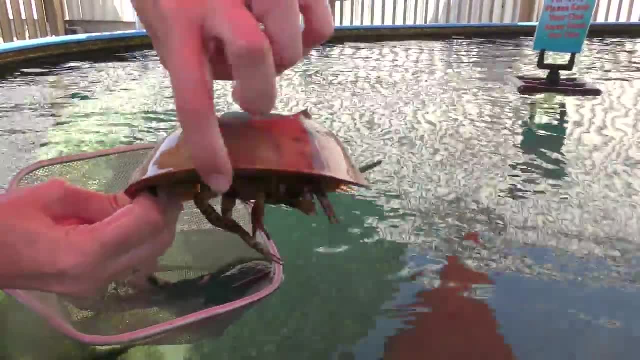 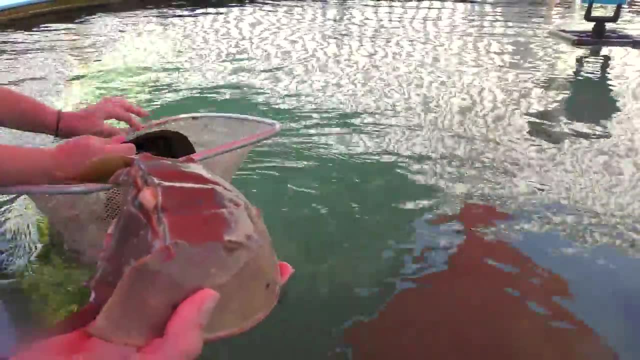 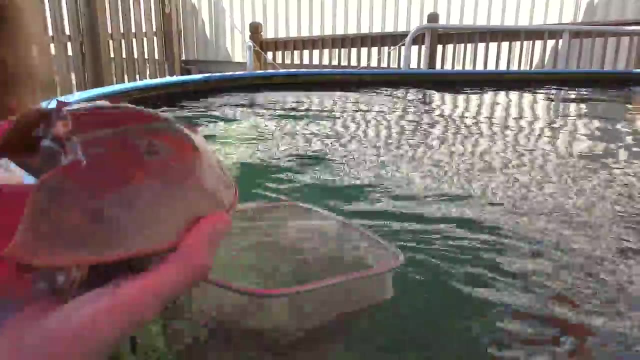 of the female is fairly flat. in the front, There's not much of an arch, And so we'll contrast that to the male in just a second. All right, We ready to bring him out, So you can see. our male's been through a little bit. Can I swap out with you? 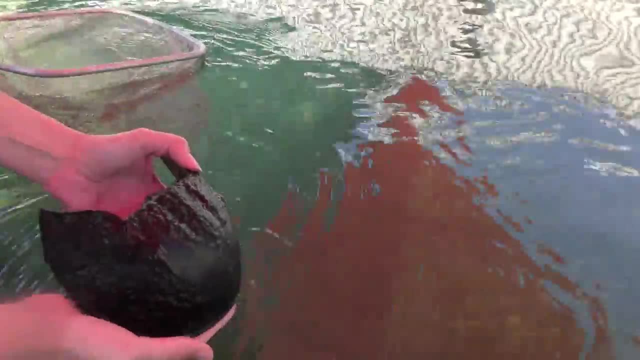 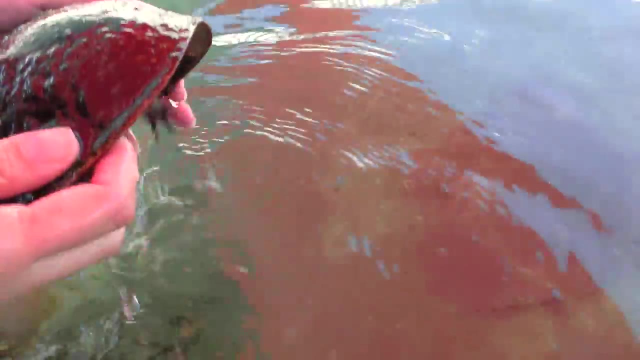 Thanks. He's been through a few things here, But this is actually. You can see this better. in the water He's got algae growing all over the surface And that's pretty common. especially as the crabs get a little bit older, People like to put some algae on their flocks. They don't want that kind of. Their shells normally produce what's called an exudate, which is a slick substance that is sort of an anti-fouling substance, but that decreases as they get older. So they'll often, especially if they're kept in in aquaria. 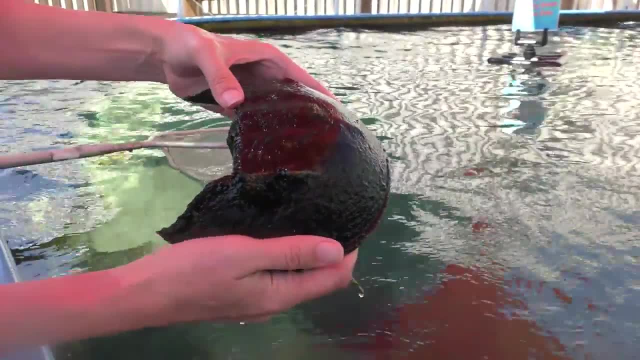 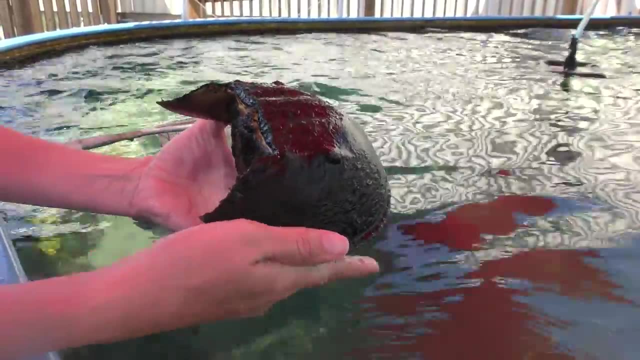 they may get some algae like this on the surface, or they may get barnacles or other kinds of animals that live on them. That's pretty common. There's actually a book even entitled Living on Limulus- all about the creatures that live on horseshoe. 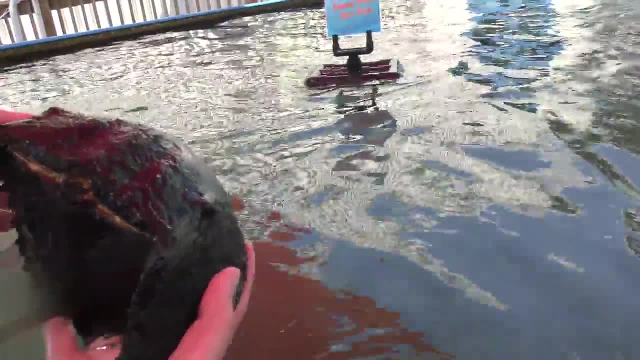 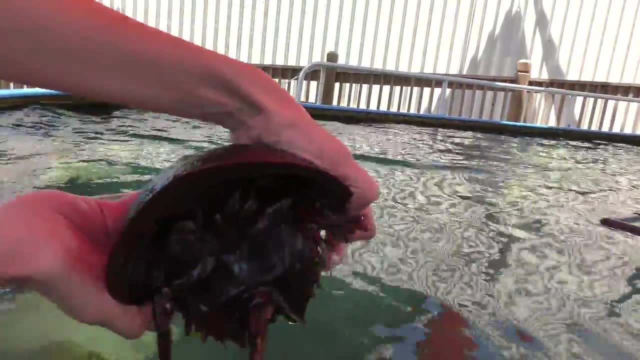 crabs and use horseshoe crabs for habitat. So you can see he's all got the same parts as the female. but we're going to flip him over and notice- actually notice- the front of his shell. See how big that arch is compared to the. 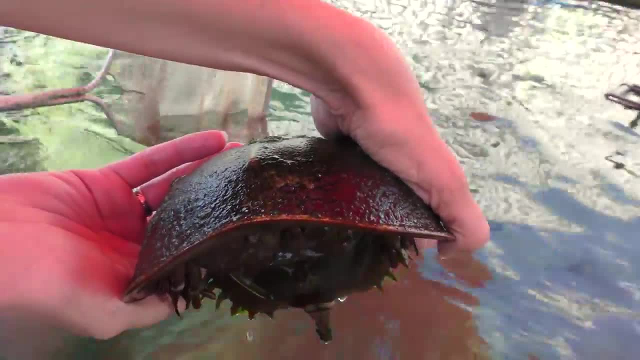 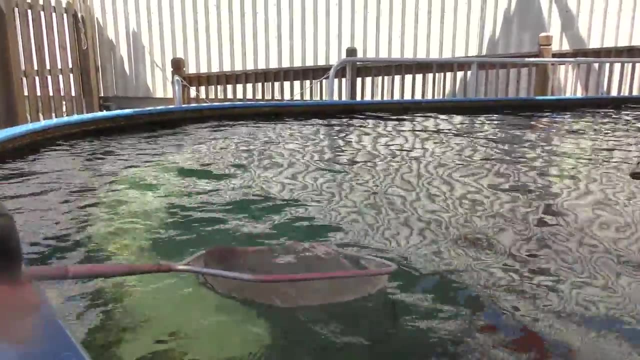 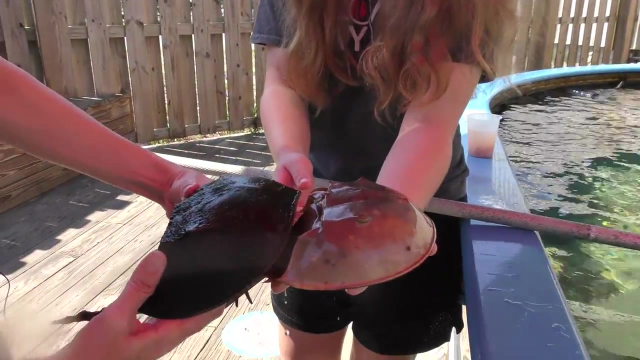 females, And that's so that he can accommodate her body when they're mating. So if we compare him to the female, Do you have her All right? I just want to show how this would work. So in mating, the male will actually amplex or hook on to. 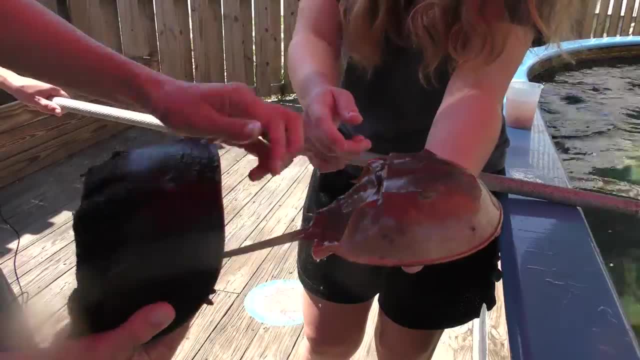 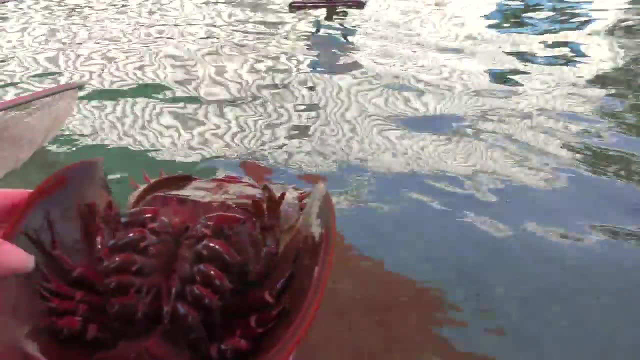 the female this way, and so he has that higher prosomal arch arch to accommodate her back, And then he'll hook on. He's got special front legs. So if you notice we flip him over, he looks just like her, Except his front legs, instead of being all pincers like 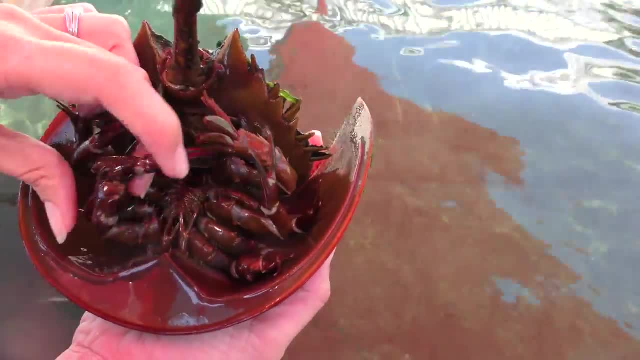 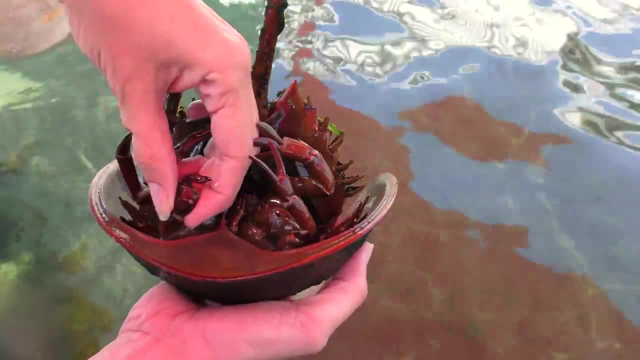 hers. see how these are pincers. His front legs are these little boxer claws. And these little boxer claws are especially modified. He doesn't like me. They're especially modified to grab onto that female shell during mating. They look like little fists. All right, And then he's also got.